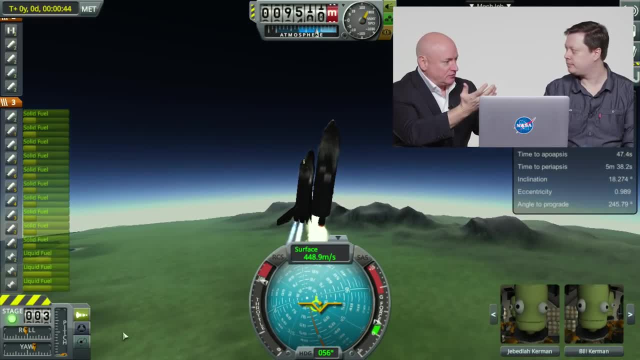 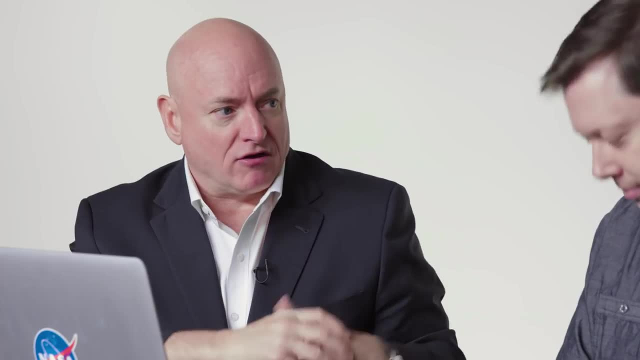 Engines will throttle down to avoid getting too high of a max dynamic pressure and then they'll throttle back up and the common call you'll hear on the ground is: go at throttle up. You don't fly this hands-on. The computer does the assembly right. 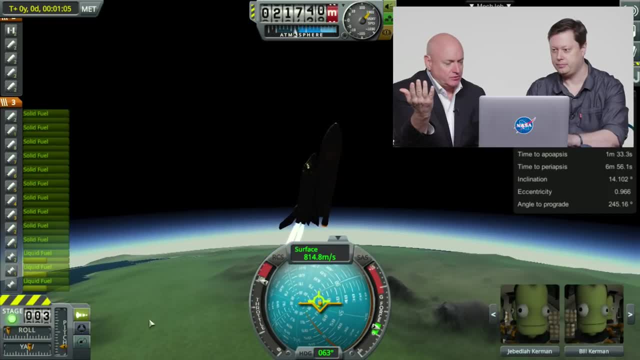 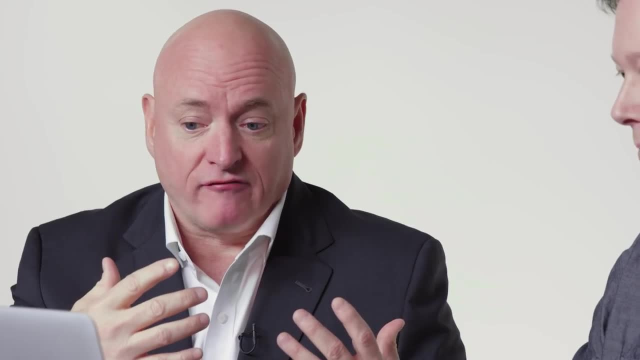 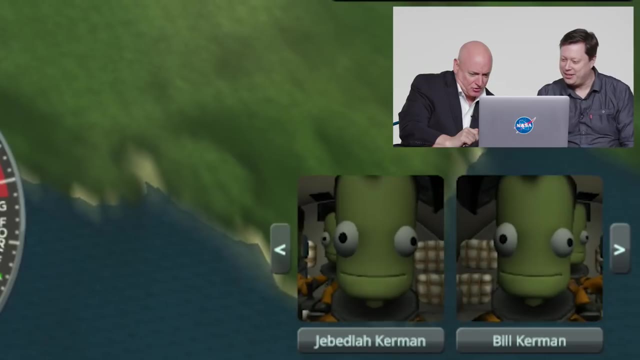 Yeah, the computer flies the space shuttle to space in an emergency. If you had issues with the control, you can take over manually after 90 seconds. And I want to point out that this Jebediah Kermin looks like my brother a little bit. 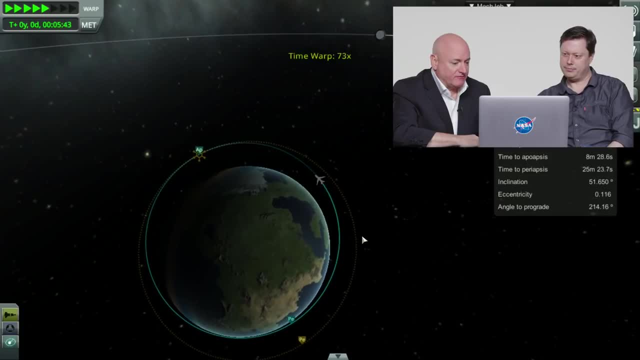 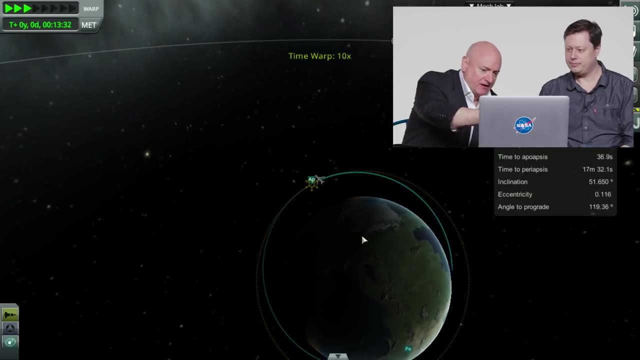 So apogee is the highest point in your orbit, the furthest away from the surface, and perigee is the lowest point in your orbit. So in this case we are at apogee and if we were going to circularize our orbit, 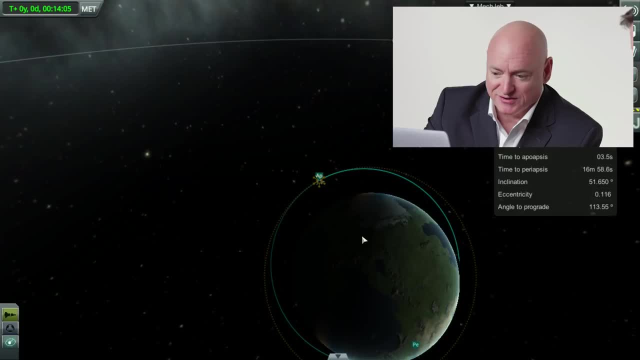 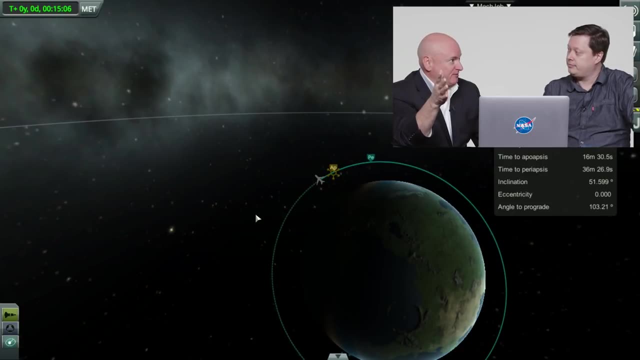 the best way to do it. I think the most fuel-efficient way to do it is to do it at apogee. Actually, the space shuttle has two, Two ohms burns generally. The first one is to give you a little bit more delta-v to get to orbit. 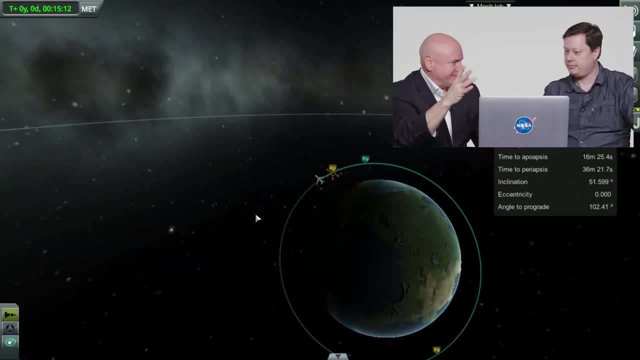 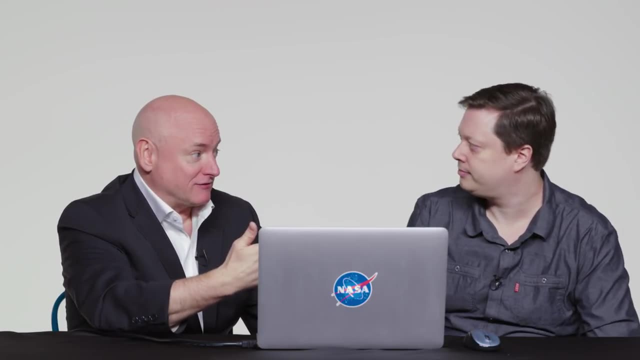 The second one is the one that's done at your apogee or pretty close to it, which then circularizes your orbit. So, instead of coming back and re-entering the Earth's atmosphere, you're in more of a circle versus an ellipse. 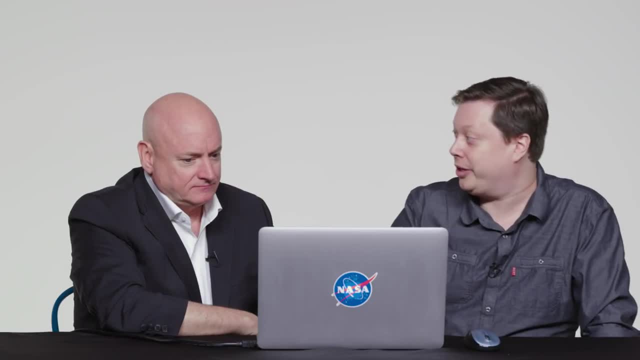 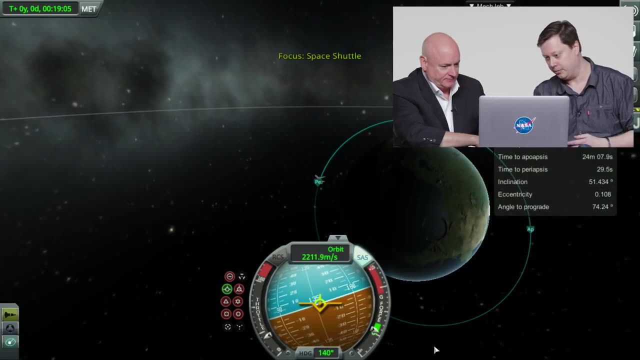 Now we can kind of demonstrate that a little bit by changing our orbit here. If I apply a little bit of thrust here, Mm-hmm, and then we pop back and look at our orbital map, we can see already. Oh yeah, look at that. 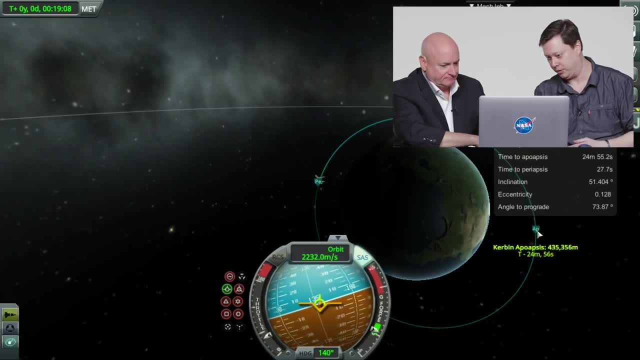 immediately opposite us. this is our period of. I'm actually piling on probably more delta-v than I want at this point. We're applying more eccentricity to our orbit. I guess We're making it more and more egg-shaped, basically. 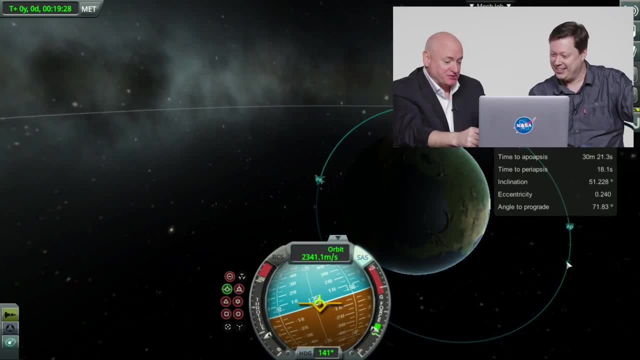 Eccentric. There you go, Which also means we're slowing down. so as our orbit gets bigger, our speed again counter-intuitive. We've added energy to the system. You would think that would make you go faster, but really what it does is it makes you go higher. 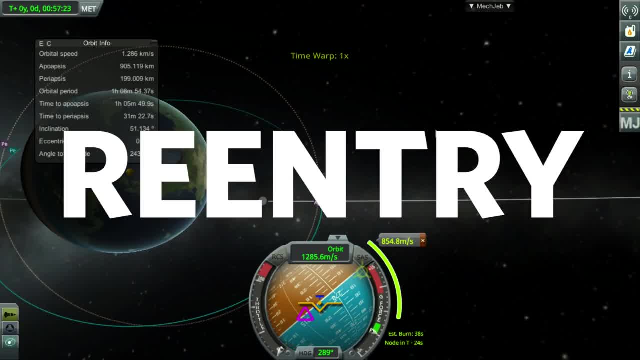 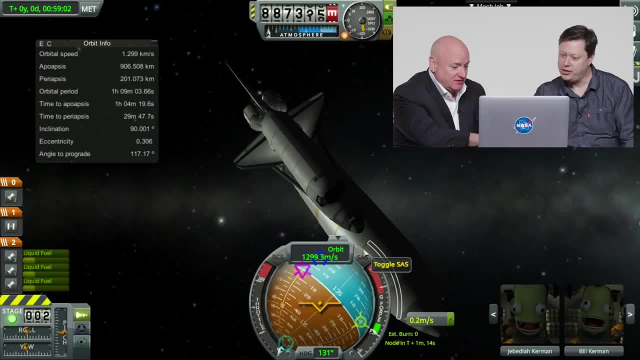 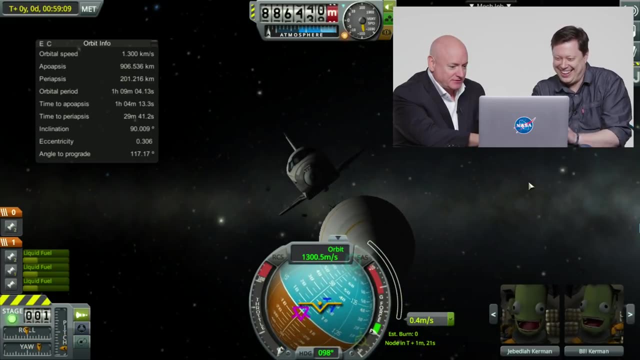 Yes, Which in fact then makes you go slower. NASA could probably use this to teach future astronauts orbital mechanics. Actually, I forgot to dump our external tank. Let me do that real quick. Man, that is a fatal error. Look at you, You are crashing. 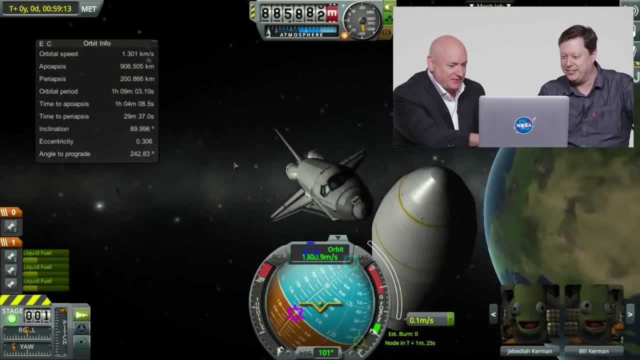 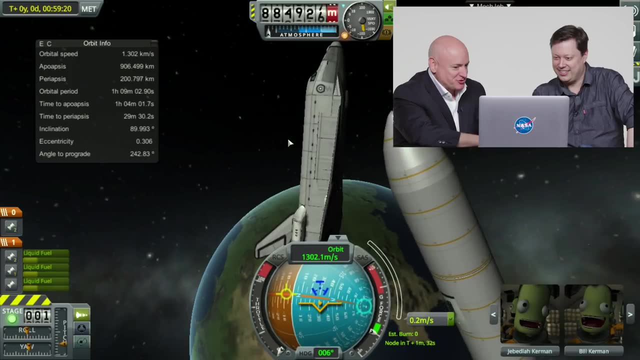 Wait a minute, wait a minute, We are crashing. No, no, we're fine, It's fine, It's all fine. You bounced off of it, That's okay. The orbiter can do that. This little nose cap there on the space shuttle. you just crushed it. 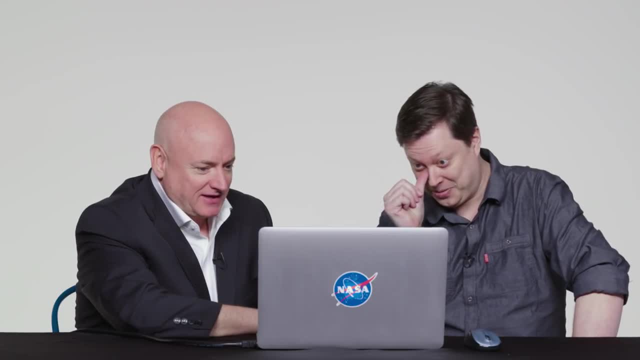 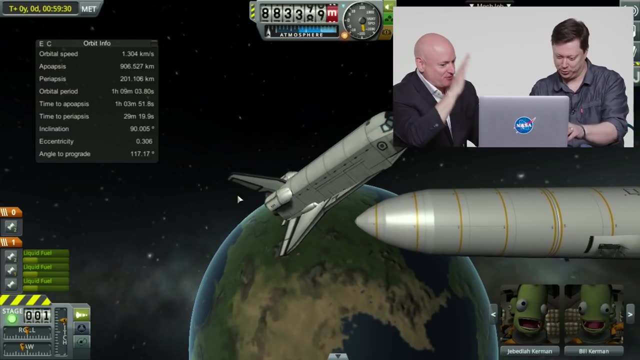 I think I may have. I may have Look at that, I may have scraped our tiles a little bit, Holy cow. Well, I, I, I punched the explosive bolts without any. I guess we could probably try to go somewhere a little bit. 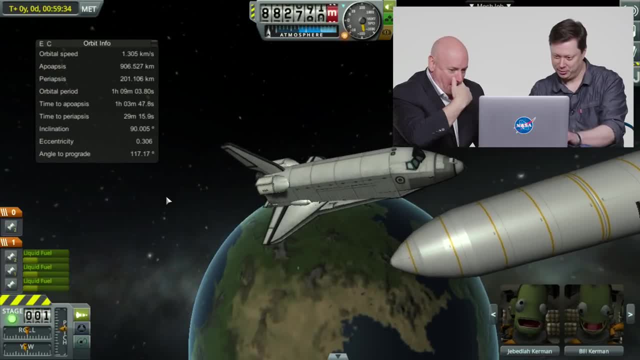 Let's see here, Let's let's see if I can give us a little bit of a, a little bit of a separate. oh boy, hold on, Wait, wait, wait, wait, wait. Ah, there we go, We're fine, We're fine. 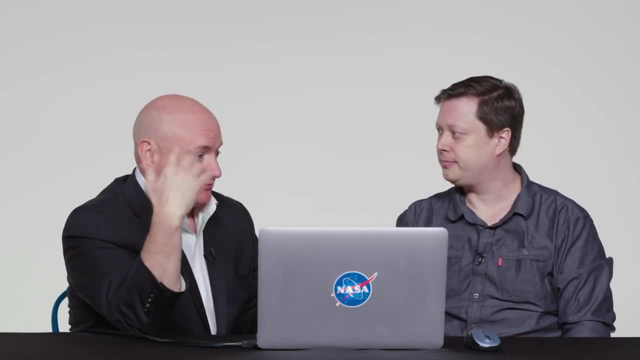 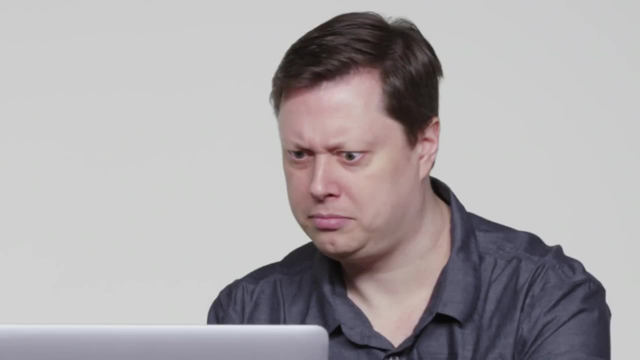 Yeah, so the way the space shuttle, or really you know the Soyuz or you know spacecraft, come back to Earth is you only have to change your orbital velocity by a few hundred miles an hour. Sure, So what happens on both the shuttle and the Soyuz case is you fire an engine so you turn around backwards. 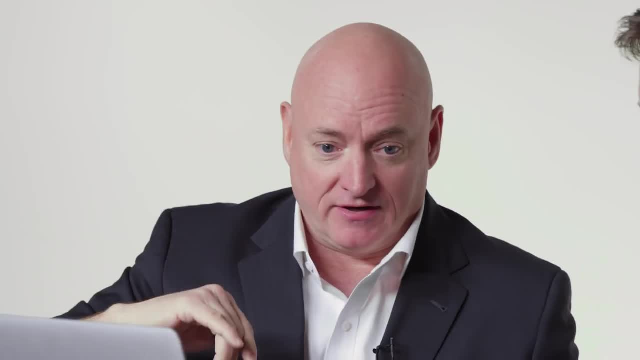 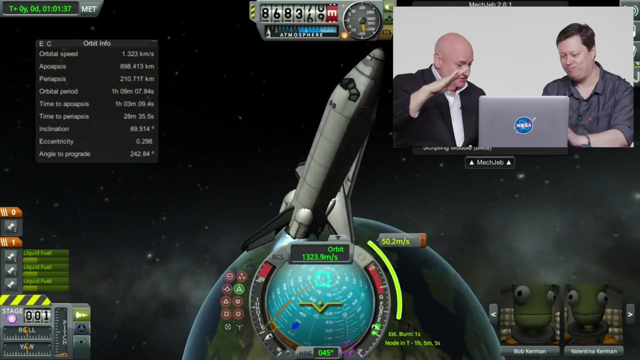 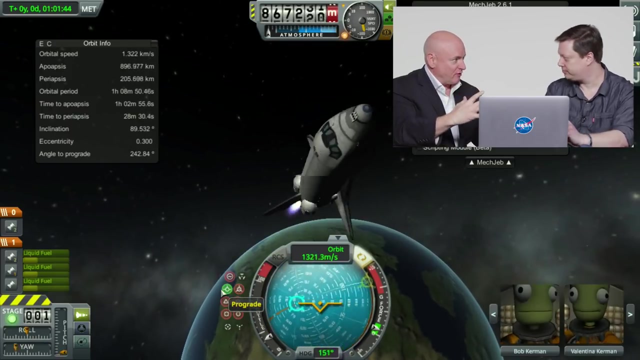 So now you're going, you know, instead of going pointy end forward, you're going pointy end backwards. Then you fire those engines to slow down and the rest of your velocity is removed from the spacecraft with friction in the atmosphere in the form of heat. 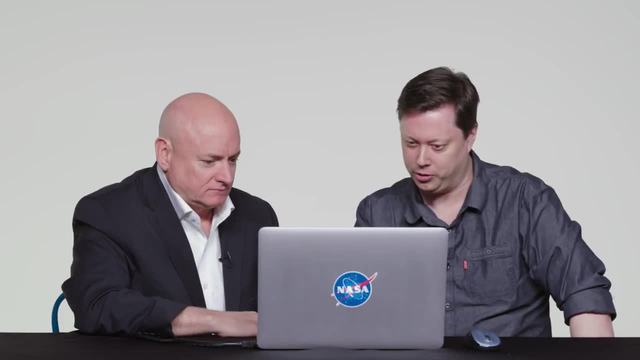 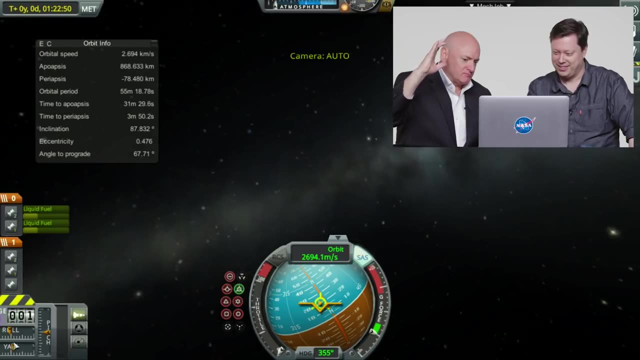 So I was going to try, Scott, to bring us into landing here. Our orbital, our ground speed is increasing rapidly. Well, just get us into the atmosphere. Okay, done We can. we can then just blow the hatch, Done. 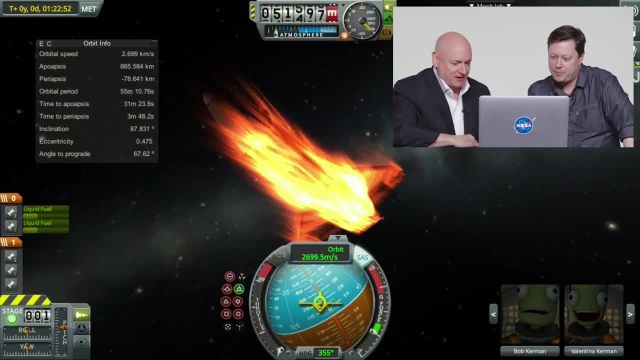 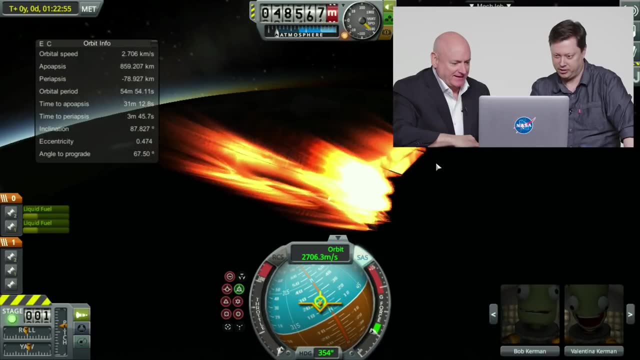 And we'll jump out and hopefully survive under our parachutes. Oh, I forgot to flip us around pro grade. So we're actually we're entering Ooh back in first. Yeah, technically I'd call this an ass in first reentry. 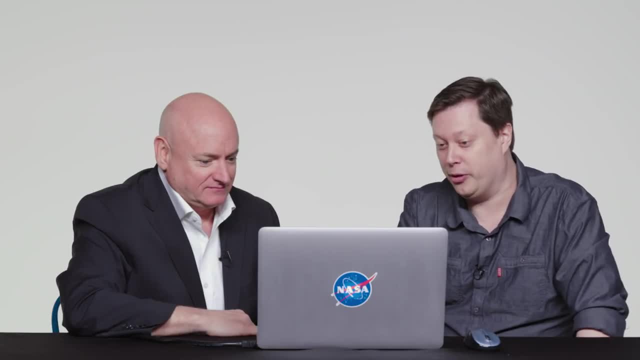 All right, Scott. Well, this has been an excellent demonstration of why you're an astronaut and I'm not. How was that for you? How close to real life was that for you, and did you enjoy it? It was exactly like real life. 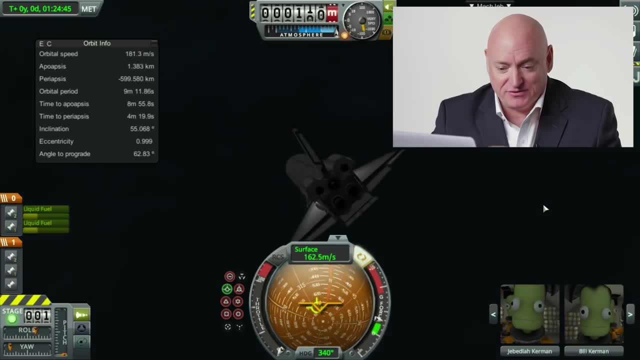 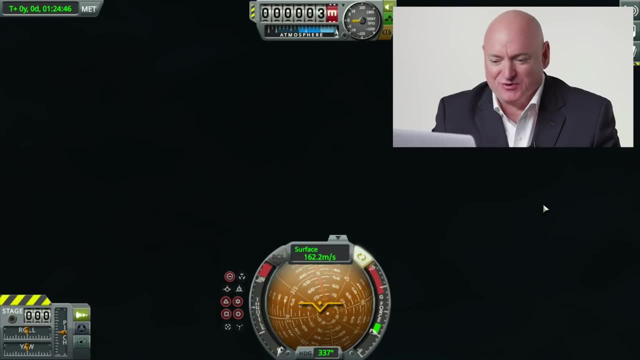 No, actually I'm just kidding. It was good You know it was. I think it's something that NASA could use to train like future flight controllers and astronauts a little bit more about orbital mechanics. I wanted to give a quick shout out to Simone Riboldi of the YouTube channel Simon and Simon. 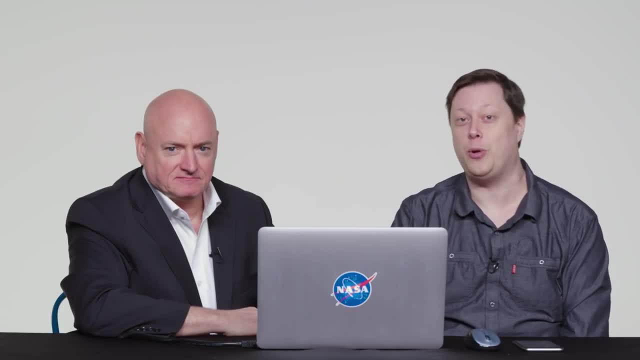 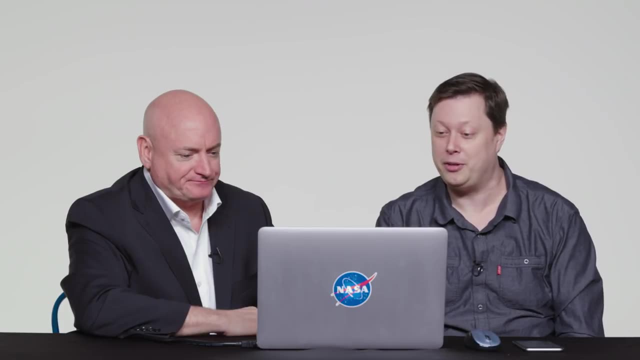 Thank you for preparing some of the Kerbal Space Program stuff for us today. We really appreciate it. Thank you also to SQuAD, the Kerbal Space Program developers, for helping us out to make this demonstration happen. Thank you, Much appreciated folks.